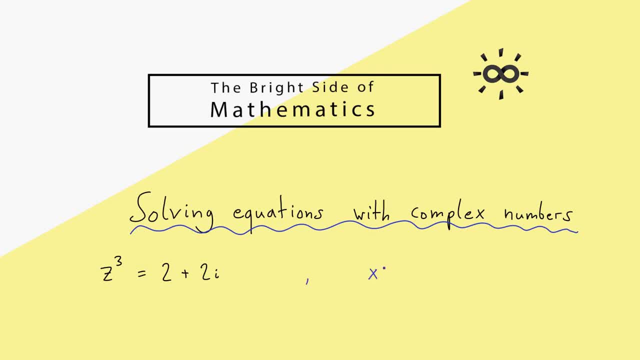 go back to the real numbers. How can you solve an equation, maybe of the form x squared equals to a fixed real number, And maybe the easiest one would be four here Now you learned, for example, in school that we have indeed two solutions here. A positive solution i could call x1, which is two. 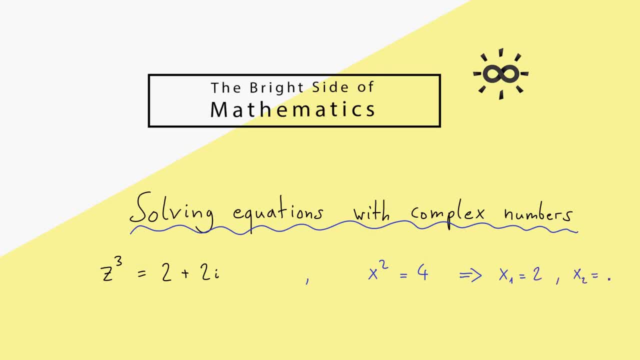 and a negative solution, which we call x2, which is minus two. So exactly two solutions. and now let's see how this looks like in the real number line. The line represents all real numbers and now i can put zero, maybe here. And now i see that my two solutions, here x2 and here x1. 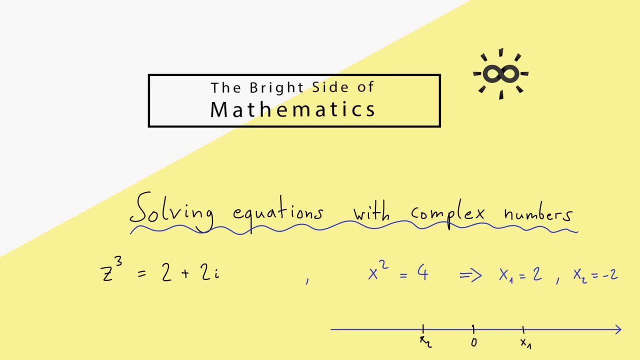 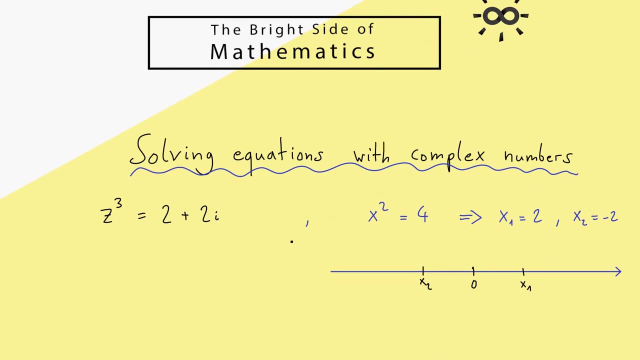 have the same distance from zero. Also, you recognize the order. We have a smaller solution and a bigger solution, Or in other words, we have a positive solution and a negative solution. And now you already know that we can't have this nice order in the complex numbers as well. 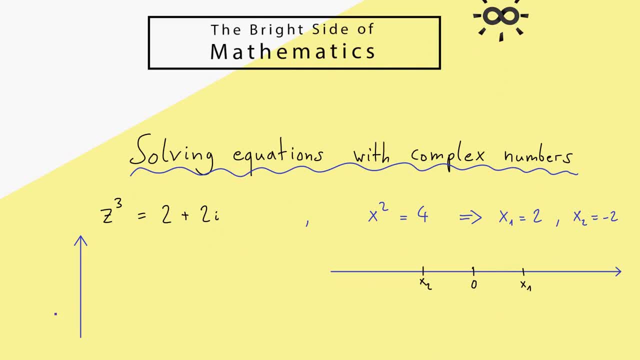 Because here now we have the whole complex plane. We have the real part on the x-axis and the imaginary part on the y-axis, And the first part we immediately see is, when we have zero again here in the middle, that we have more numbers that have the same distance from zero, For example for this: 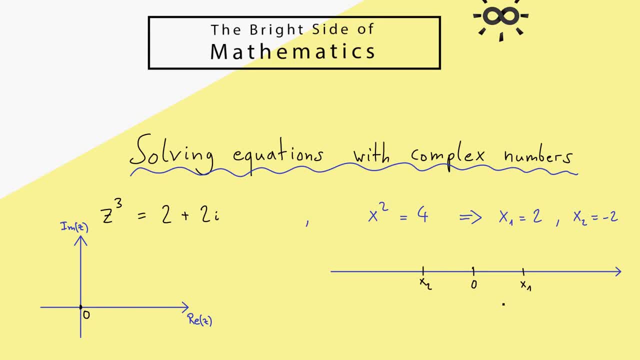 distance two. we only have two numbers in the real number line but immediately infinitely many in the complex plane, because it describes a circle around zero with radius two. Also we don't have an easy distinction between left and right as in the number line, so we can't say we have a positive or 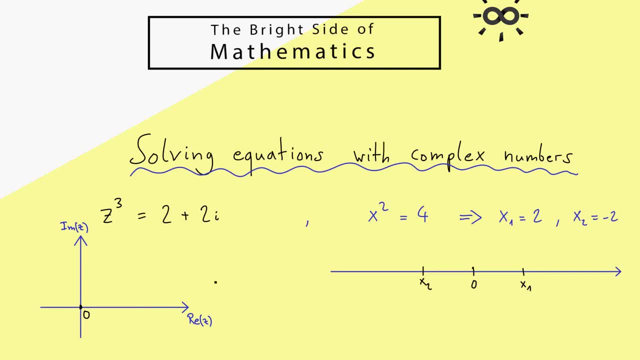 negative solution here in the complex plane. Hence we need another picture in the complex plane, and that is what i will do later. First, i want some visualization for this complex number here, so i put this in the complex plane. So we have two here and the same way we have two here. This means the complex number with real part. 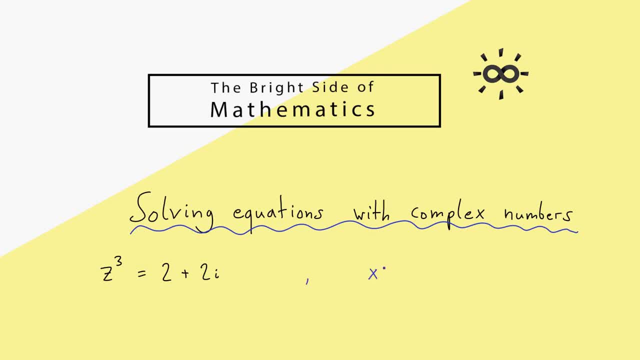 go back to the real numbers. How can you solve an equation, maybe of the form x squared equals to a fixed real number, And maybe the easiest one would be four here Now you learn for example in school that we have indeed two solutions here. A positive solution i could call x1, which is two. 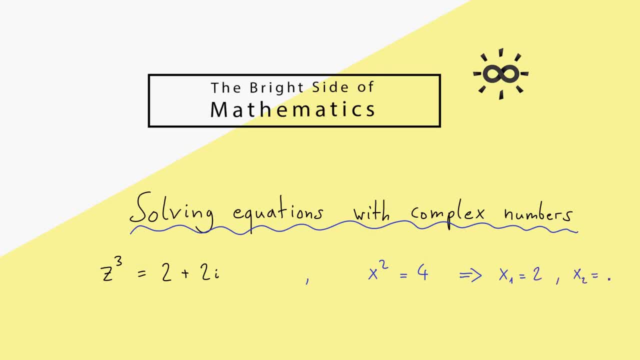 and a negative solution, which we call x2, which is minus two. So exactly two solutions. and now let's see how this looks like in the real number line. The line represents all real numbers and now i can put zero, maybe here. And now i see that my two solutions, here x2 and here x1. 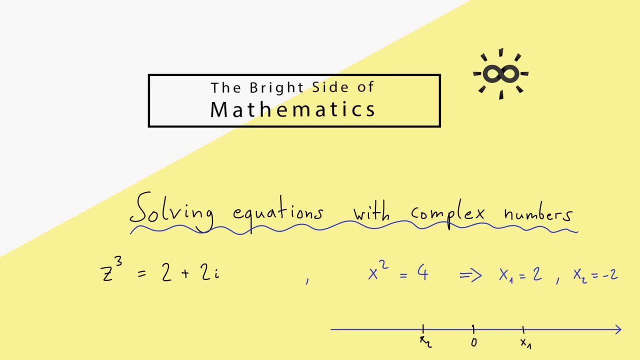 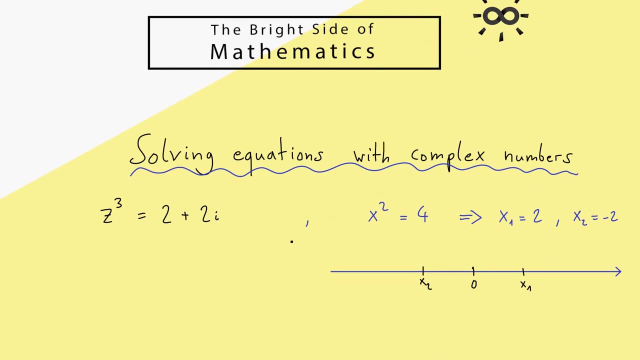 have the same distance from zero. Also, you recognize the order. We have a smaller solution and a bigger solution, Or in other words, we have a positive solution and a negative solution. And now you already know that we can't have this nice order in the complex numbers as well. 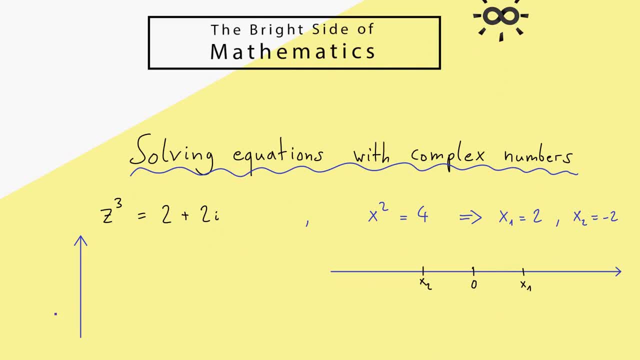 Because here now we have the whole complex plane. We have the real part on the x-axis and the imaginary part on the y-axis, And the first part we immediately see is, when we have zero again here in the middle, that we have more numbers that have the same distance from zero, For example for this: 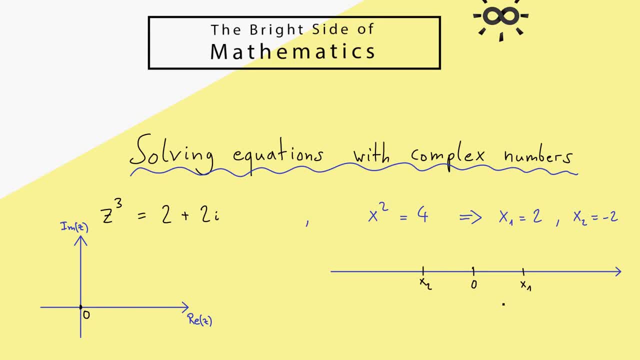 distance two. we only have two numbers in the real number line but immediately infinitely many in the complex plane, because it describes a circle around zero with radius two. Also we don't have an easy distinction between left and right as in the number line, so we can't say we have a positive or 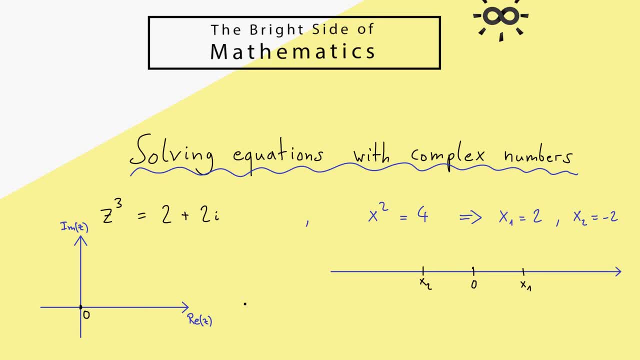 negative solution here in the complex plane. Hence we need another picture in the complex plane, and that is what i will do later. First, i want some visualization for this complex number here, so i put this in the complex plane. So we have two here and the same way we have two here. This means the complex number with real part two. 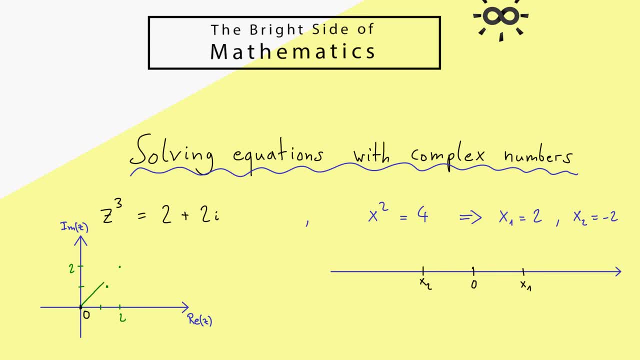 two, and imaginary part two lies here, so we can visualize this with an error that goes to this point. One important thing i can immediately tell you now is if you have an exponent, so a power of set here, then it's always helpful to rewrite this number on the right. You should rewrite it in the polar form or better, in the. 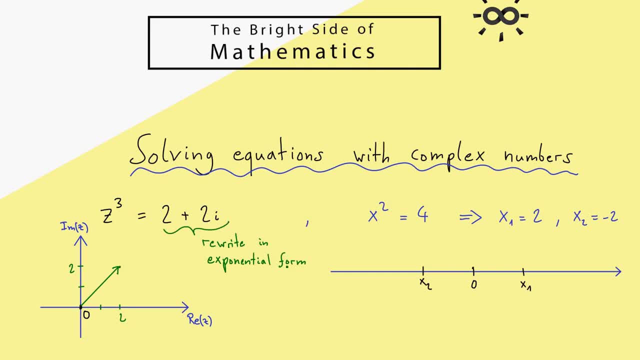 exponential form. You will see soon that this is indeed very helpful. Okay, so we describe our complex number here now with two things: First, the distance from zero, which means the absolute value, and second, the angle from x-axis to the vector itself In order to calculate these two things. 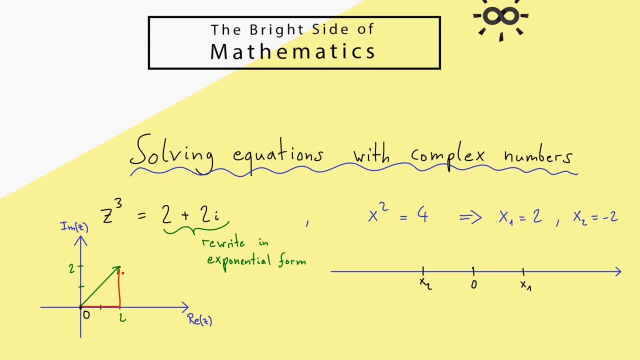 you can just draw this, The right angle triangle here, and then you know you can calculate the length of this side by using pythagoras theorem. And to calculate the angle here, which i call phi, now, you can use a trigonometric function. Most of the time one uses the tangent, because then you can immediately use the y. 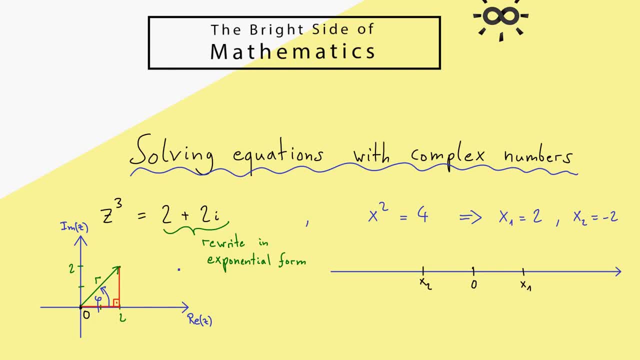 coordinate and the x coordinate. However, in our example we don't have to calculate at all because we immediately see that we bisect the right angle here. So we cut pi over 2 in half, which means we get phi as pi over 4, which means 45 degree Just as well, we also get our absolute value, which i 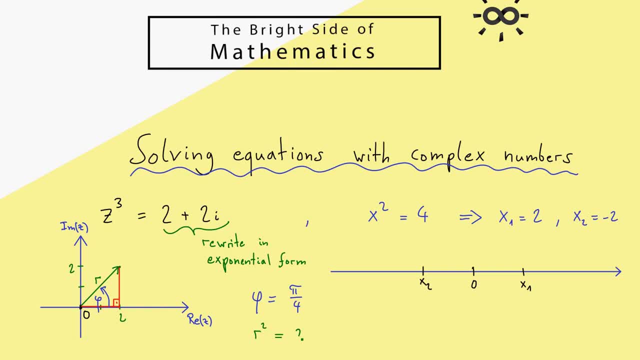 called r. By using pythagoras, we know now: r squared is equal to 2 squared plus 2 squared, which is 8.. Now r is of course the positive solution here, so r is equal to the square root of 8.. Now, to summarize this, we can rewrite our complex number 2 plus 2i in an exponential form: 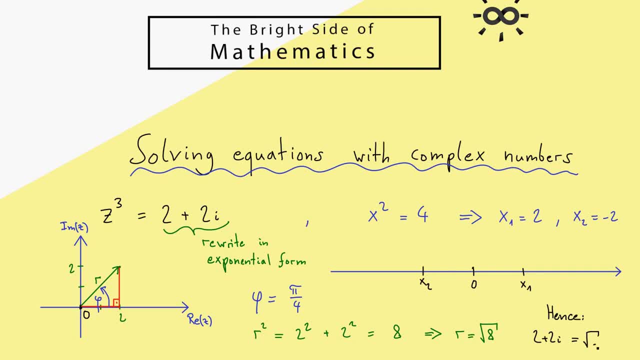 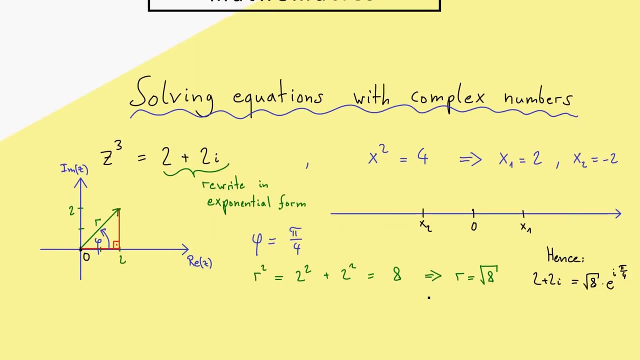 We have now the number equal to, first the absolute value r, and then times e to the power i, and then comes the angle, phi, which is, in our case, pi over 4.. Okay, so this is the exponential form, and this is always helpful when you consider powers in an. 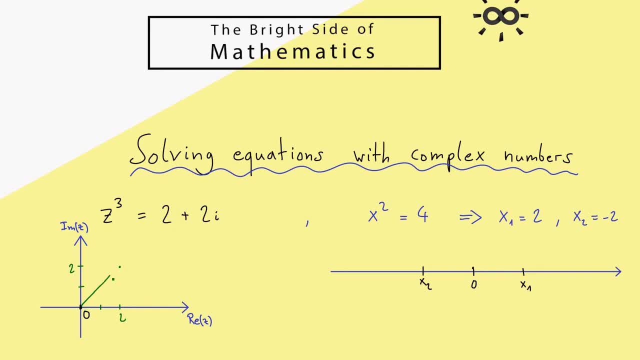 and imaginary. part two lies here, so we can visualize this with an error that goes to this point. One important thing i can immediately tell you now is if you have an exponent, so a power of set here, then it's always helpful to rewrite this number on the right. You should rewrite it in the polar form or better, in the. 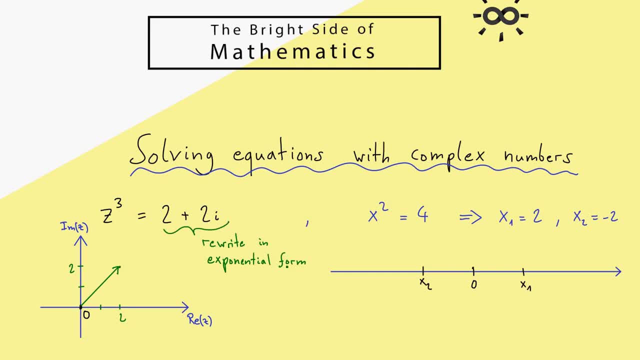 exponential form. You will see soon that this is indeed very helpful. Okay, so we describe our complex number here now with two things: First, the distance from zero, which means the absolute value, and second, the angle from x-axis to the vector itself In order to calculate these two things. 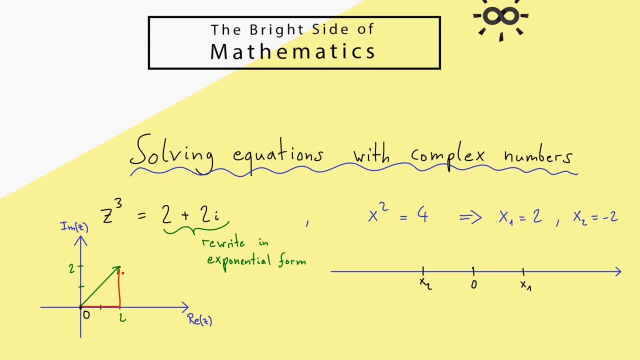 you can just draw this, The right angle triangle here, and then you know you can calculate the length of this side by using pythagoras theorem. And to calculate the angle here, which i call phi, now, you can use a trigonometric function. Most of the time one uses the tangent, because then you can immediately use the y. 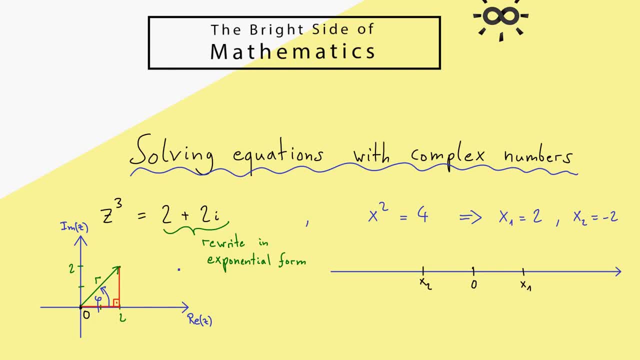 coordinate and the x coordinate. However, in our example we don't have to calculate at all because we immediately see that we bisect the right angle here. So we cut pi over 2 in half, which means we get phi as pi over 4, which means 45 degree Just as well, we also get our absolute value, which i 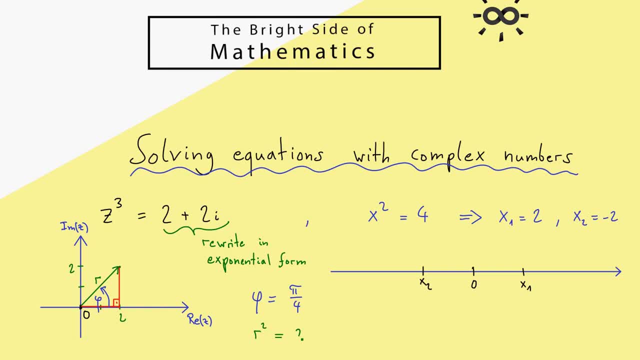 called r. By using pythagoras, we know now: r squared is equal to 2 squared plus 2 squared, which is 8.. Now r is of course the positive solution here, so r is equal to the square root of 8.. Now, to summarize this, we can rewrite our complex number 2 plus 2i in an exponential form: 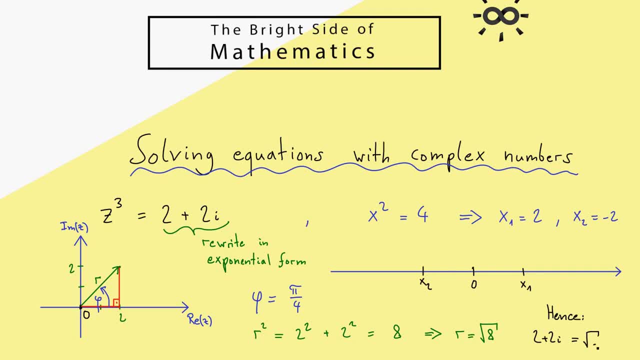 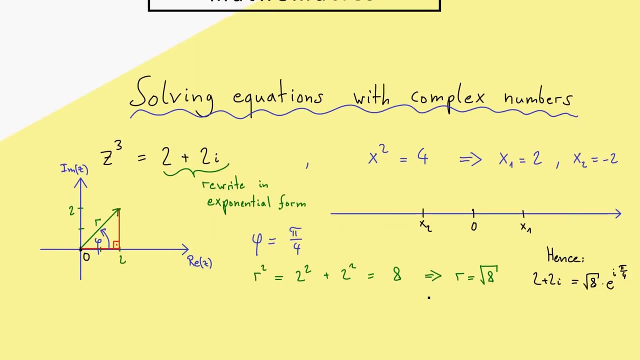 We have now the number equal to, first the absolute value r, and then times e to the power i, and then comes the angle, phi, which is, in our case, pi over 4.. Okay, so this is the exponential form, and this is always helpful when you consider powers in an. 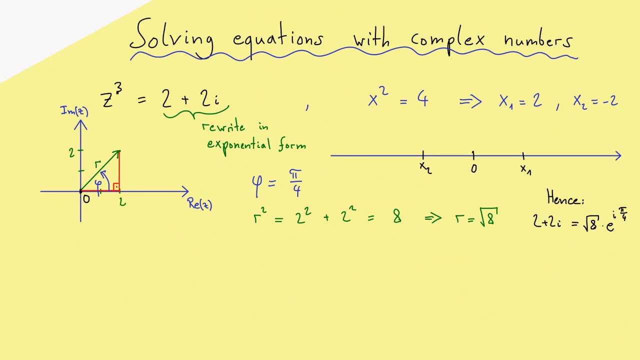 equation, because calculating with exponents is much easier. when you have the exponential function here In this case, then you can just multiply the exponents, and then it does not matter how big this power is indeed, because you just have to multiply them. Well, and now we can solve our equation from. 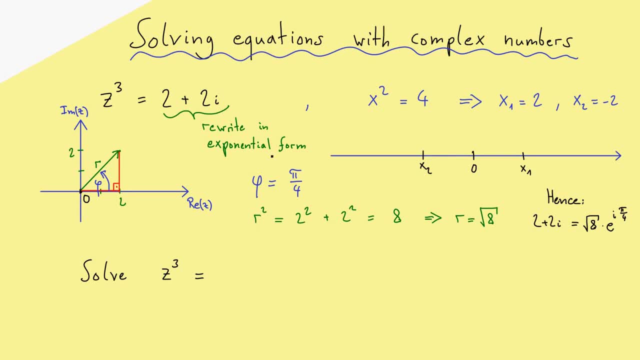 the beginning. Still, we have z cubed, but the right hand side is now much easier. Now my first advice here is that you should rephrase that a little bit. Namely, you use the fact that we don't change our complex number if we add a full turn, which means we add 2 pi to our angle. here 2 pi is the full circle. 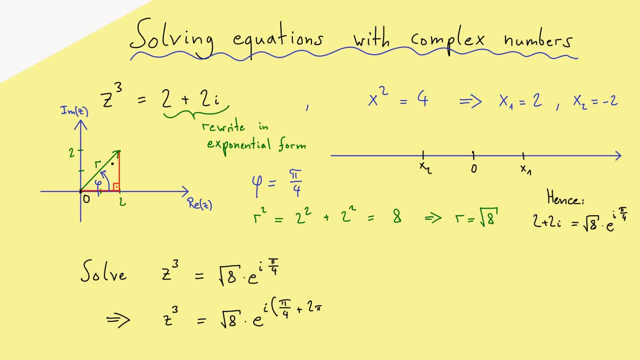 so we end up at the same point in the complex plane. Now we still get to the this point by writing this complex number, or, in other words, this is just another representation of the same complex number from the beginning. However, at this point we can do even more, because 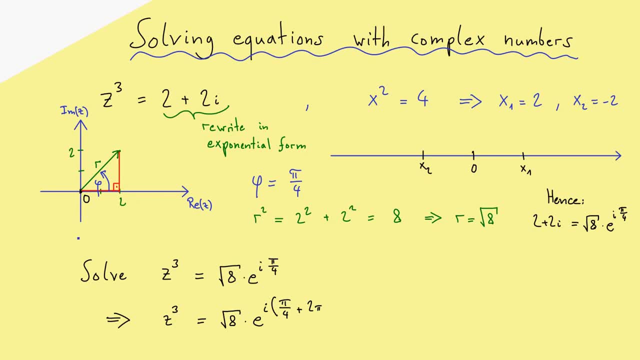 if we can add one turn, we also can add two turns and even three and so on. We still end at the same complex number in the complex plane. In short, we can add k turns, so k times 2 pi. Therefore we can choose as many turns as we want. so we can choose our k, maybe first as zero, which? 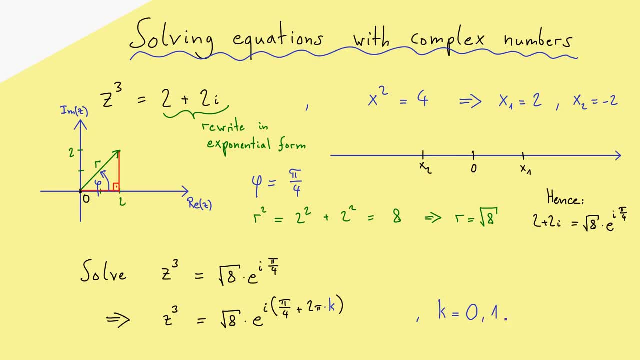 is this representation from before, or one turn, or two turns, or three turns and so on? Okay, now, before we go further, we should first answer the question: how many solutions can this equation have? There, it is helpful to first look back at our real example from before. There we had: 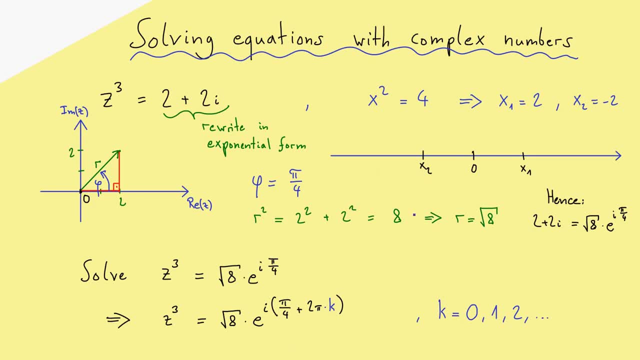 two solutions for a quadratic equation. Of course, we also can consider the equation in the complex numbers, which means we have to add the imaginary axis to our picture. here, However, we still stay at two solutions, and what we also find is that all solutions have to lie on the circle around zero. 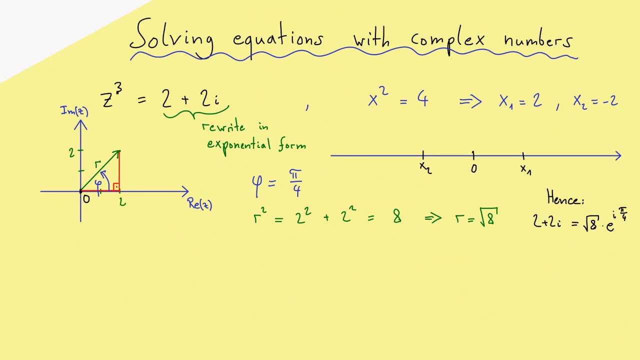 equation, because calculating with exponents is much easier. when you have the exponential function here In this case, then you can just multiply the exponents, and then it does not matter how big this power is indeed, because you just have to multiply them. Well, and now we can solve our equation from. 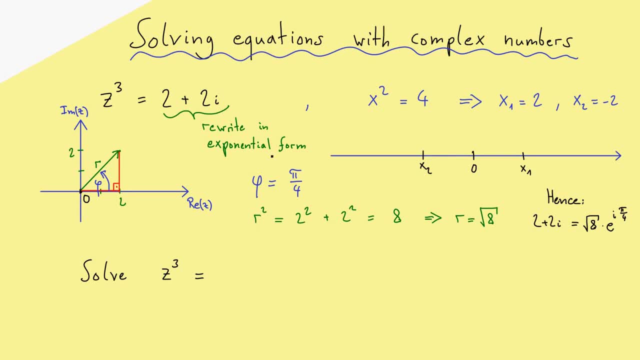 the beginning. Still, we have z cubed, but the right hand side is now much easier. Now my first advice here is that you should rephrase that a little bit. Namely, you use the fact that we don't change our complex number if we add a full turn, which means we add 2 pi to our angle. here 2 pi is the full circle. 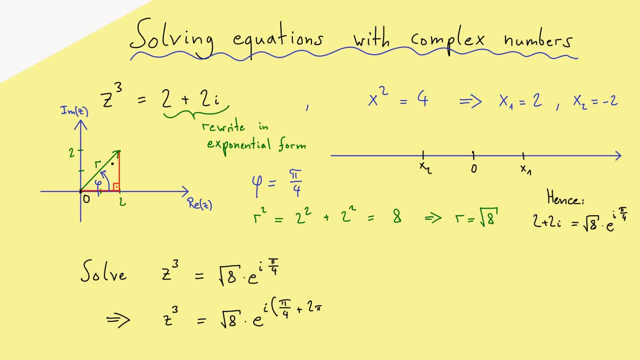 so we end up at the same point in the complex plane. Now we still get to the this point by writing this complex number, Or in other words, this is just another representation of the same complex number from the beginning. However, at this point we can do even more, because 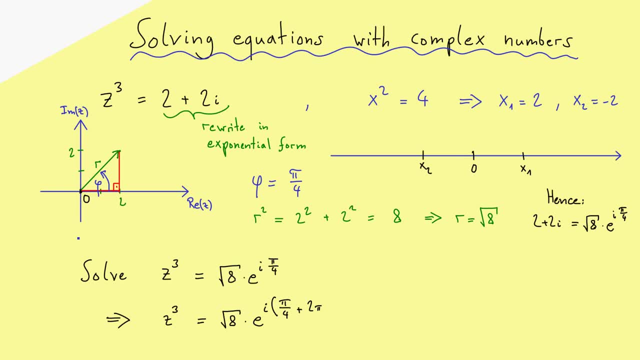 if we can add one turn, we also can add two turns and even three and so on. We still end at the same complex number in the complex plane. In short, we can add k turns, so k times 2 pi. Therefore we can choose as many turns as we want. So we can choose our k, maybe first as zero, which? 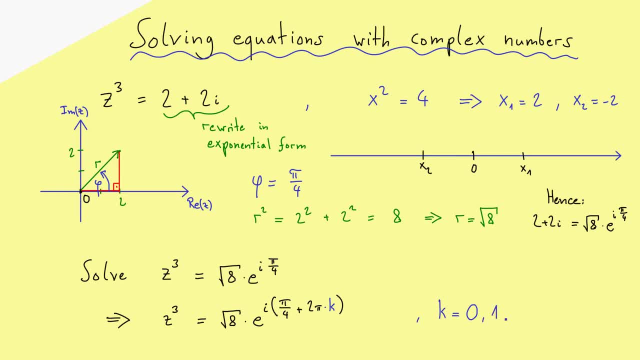 is this representation from before, Or one turn, or two turns, or three turns and so on? Okay, now, before we go further, we should first answer the question: how many solutions can this equation have? There, it is helpful to first look back at our real example from before. There we had: 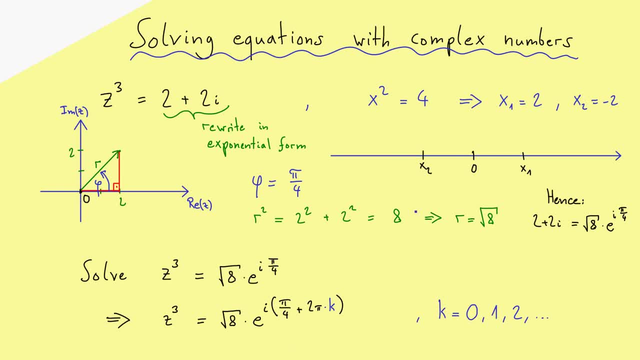 two solutions for a quadratic equation. Of course, we also can consider the equation in the complex numbers, which means we have to add the imaginary axis to our picture. here, However, we still stay at two solutions, And what we also find is that all solutions have to lie on the circle around. 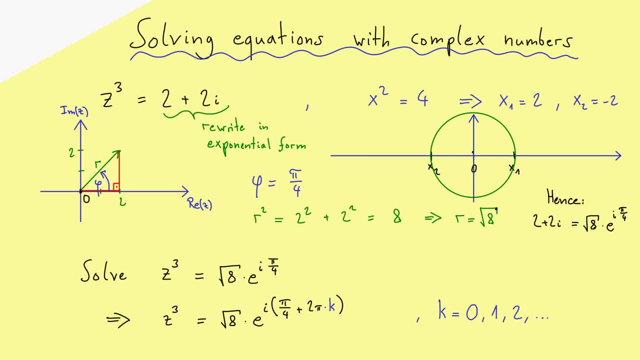 zero, which i told you at the beginning. So this is now the circle with radius two, a round zero in the complex plane. Hence, if you search for real solutions, you only have two possible points on the real line, Namely the intersections with the circle, with the line. 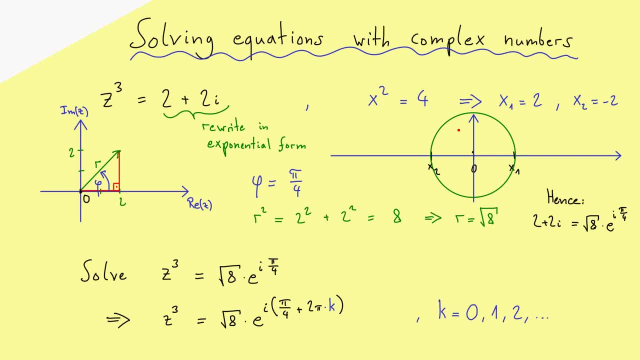 Okay, one result is: all complex solutions have to lie on this circle with the given fixed radius, And the other result is that the solutions divide this circle in same sized pieces. In this example you see this very easily. So this is the first solution, So the error to the right. Then comes one half turn and then we find: 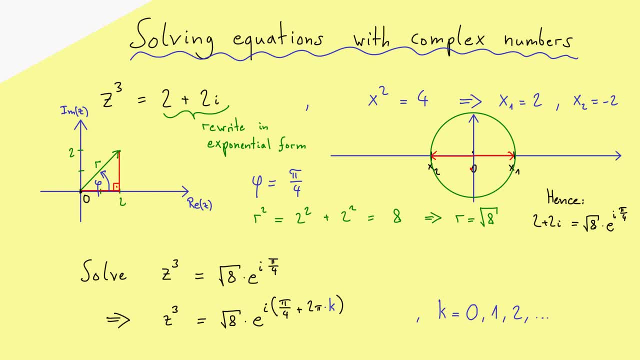 the second error to the left. So half a circle here and then half a circle here. Hence, this is what you can remember if you have the quadratic equation here, The circle is divided in two half circles, So it's cut in half. Now, in our case, with power three, we know the circle is cut in three equal parts. 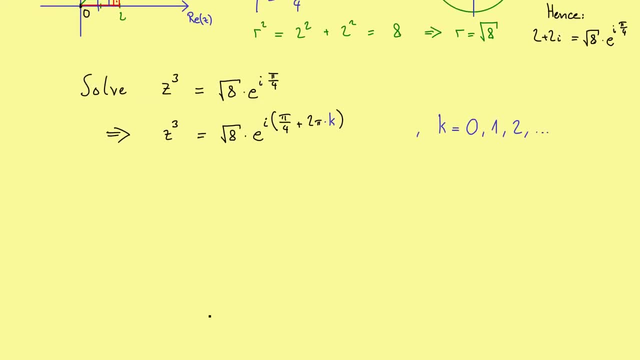 In the same way, if you have a power of four, you cut the circle in four equal parts, and so on. Hence, please remember, the exponent here gives you the number of solutions on this circle. So when we're here, it's not so hard to see. And let's draw the circle in this case again. 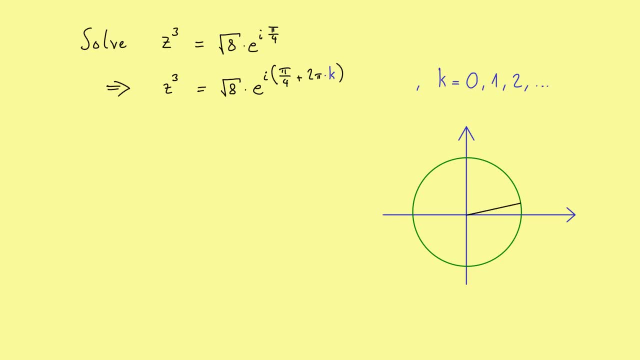 So maybe let's put in the assumption that we have found one solution, So maybe this point here. This means that this point solves this equation here And now. we find also all the other solutions, Namely, there are two, Because we know the circle. 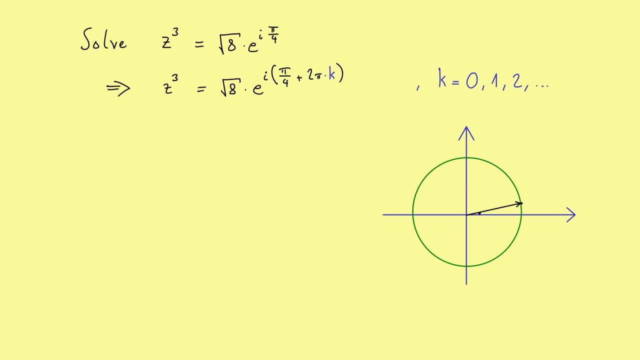 is divided into three equal parts, Which means if we go 120 degree here to the left, we find this error. And then we go 120 degree in the positive direction here and we find this error. Hence this point, and this point is all the same. 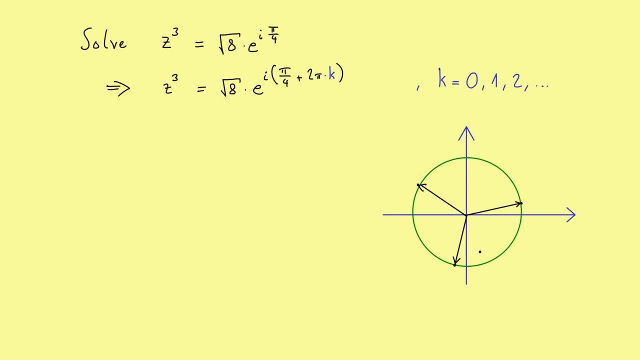 Also a solution If we now go further. so if you add again 120 degree, you end up at the first solution. Here you see, the uniform distribution on the circle is a general result that you can always use when you want to generate all the solutions from one known solution. In short, if 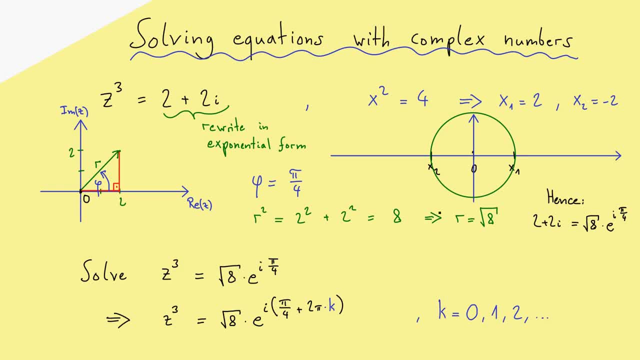 which i told you at the beginning. So this is now the circle with radius two around zero in the complex plane. Hence, if you search for real solutions, you only have two possible points on the real line, namely the intersections with the circle, with the line. 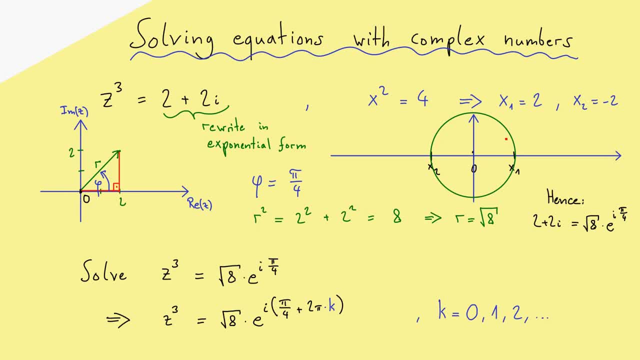 Okay, one result is: all complex solutions have to lie on this circle with the given fixed radius, and the other result is that the solutions divide this circle in same sized pieces. In this example you see this very easily. So this is the first solution, so the error to the right then comes one half turn. 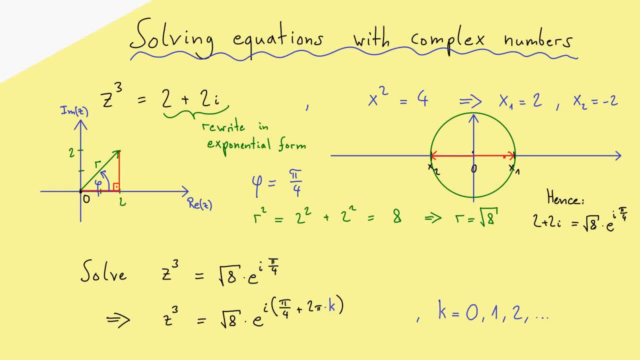 and then we find the second error to the left. So half a circle here and then half a circle here. Hence, this is what you can remember if you have the quadratic equation here, The circle is divided in two half circles, so it's cut in half. Now, in our case, with power three, we know the circle is: 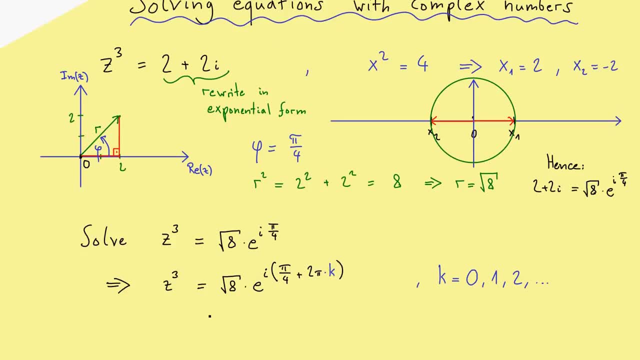 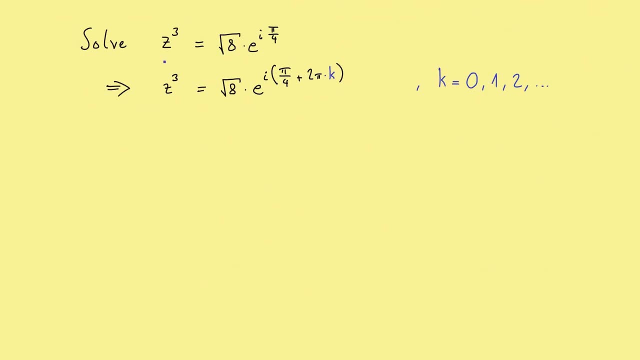 cut in three equal pieces. So this is what you can remember if you have the quadratic equation here. In the same way, if you have a power of four, you cut the circle in four equal parts, and so on. Hence, please remember, the exponent here gives you the number of solutions on this circle. 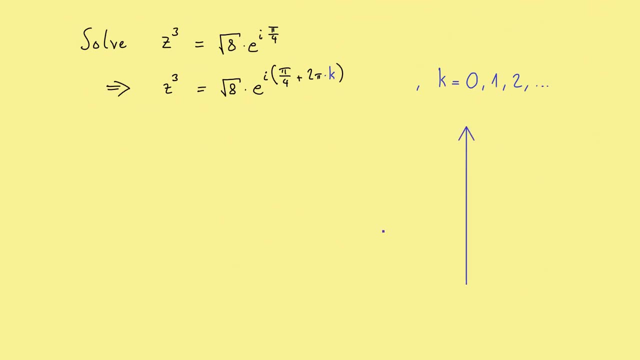 So when we're here it's not so hard to see, and let's draw the circle in this case again. So maybe let's put in the assumption that we have found one solution. So maybe this point here, This means that this point solves this equation. 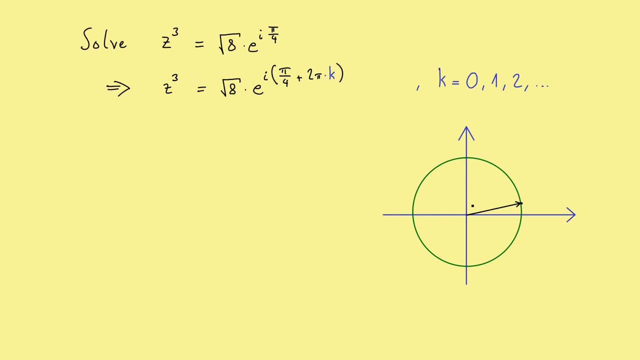 And now we find also all the other solutions. Namely, there are two, Because we know the circle is divided into three equal parts, Which means if we go 120 degree here to the left, we find this error. and then we go 120 degree in the positive direction here, and we find this error. 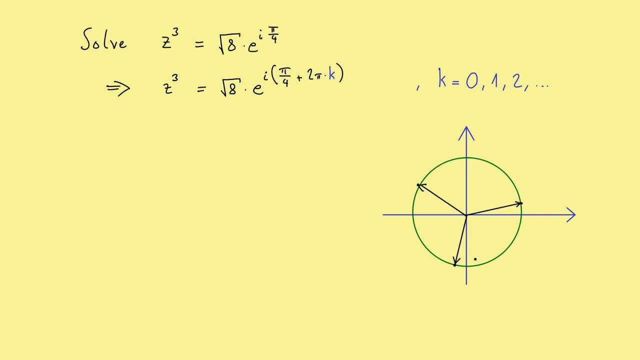 Hence this point. and this point is all the same If we now go further. so if you add again 120 degree, you end up at the first solution. Here you see, the uniform distribution on the circle is a general result that you can always use when you want to generate all the solutions from one known solution. In short, if you have one. 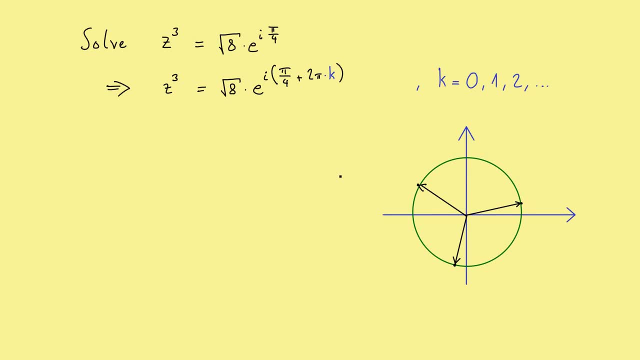 you get all the others back then And you will see that now in our calculation here on the left In a formal way, we now use the exponent 1 over 3 on both sides, and then we find indeed all the solutions, And I will count the solutions with an index k. So set index k is equal to 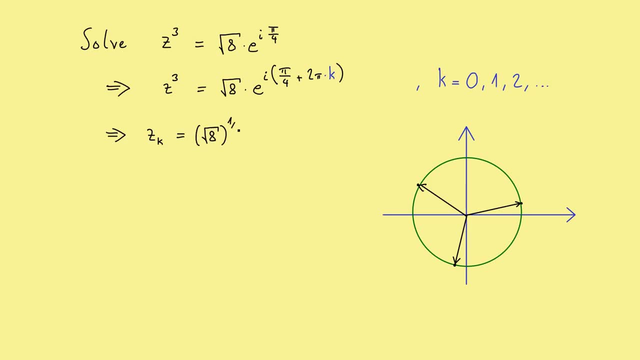 First we have the square root of 8 to the power 1 over 3 and then the exponential function to the power 1 over 3.. However, this simply means that we multiply this exponent with 1 over 3.. Ok, so let's rephrase that a little bit even more. 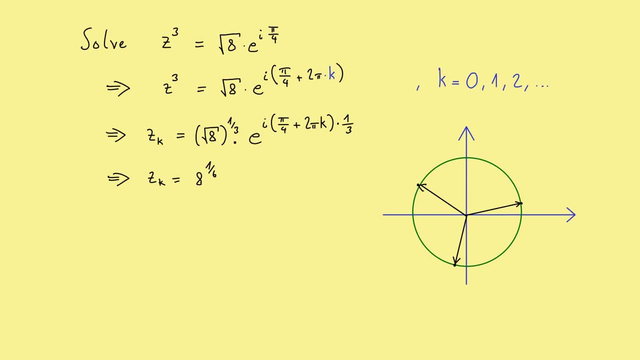 So we can write the 8 to the power 1 over 6. So combine the square root with the 1 over 3. And the same way here we do the multiplication. So we have pi over 12 plus, and there we have 2 over 3 pie times k. 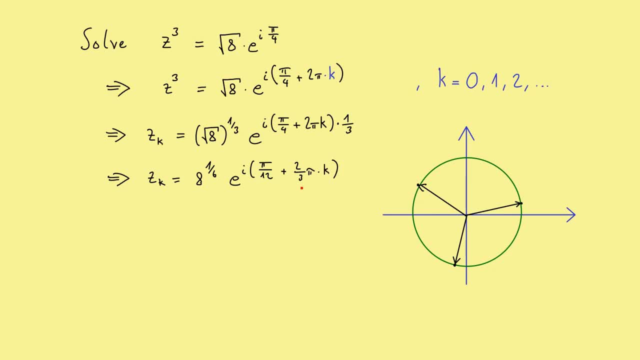 Here you should immediately recognise our 2 over 3, same truth as the 7 over 3ination equation. Our 2 over 3 pi is exactly our 120 degree. we saw earlier in our circle here And maybe you also recognize our first solution here. 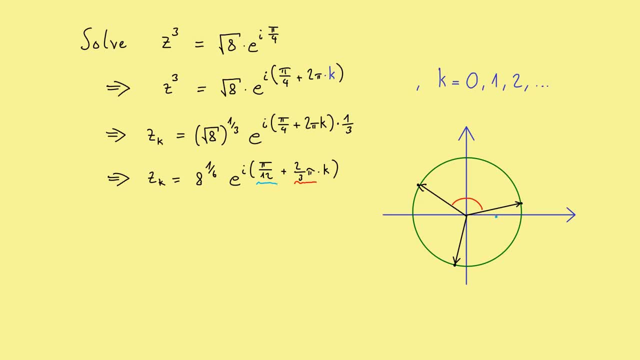 This is pi over 12, so 15 degree. This is the angle here. And this makes totally sense because now if you go to the power 3, you have to add up the angle 3 times. So 3 times this angle you end up by 45 degree. 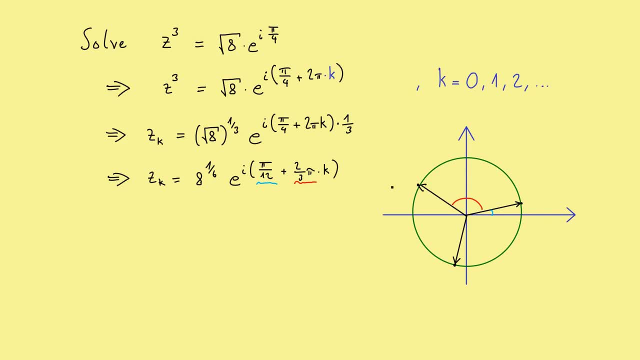 which is our original angle from the number at the beginning. So this is indeed our first solution, And we find it if we put k equal to 0. Then we find the second solution: if we add 120 degree, So this would be k equal to 1.. 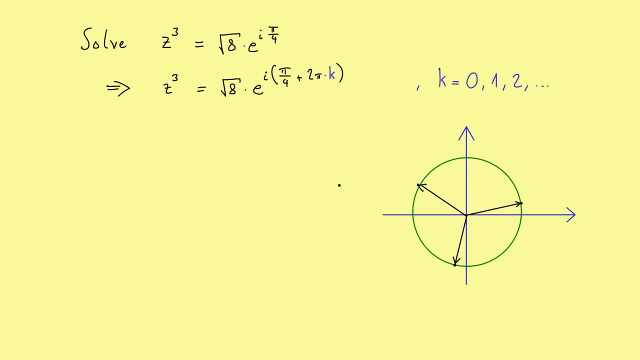 you have one, you get all the others back then, And you will see that now in our calculation here on the left In a formal way, we now use the exponent 1 over 3 on both sides, And then we find indeed all the solutions, And I will count the solutions with an index k. So set index k is equal to 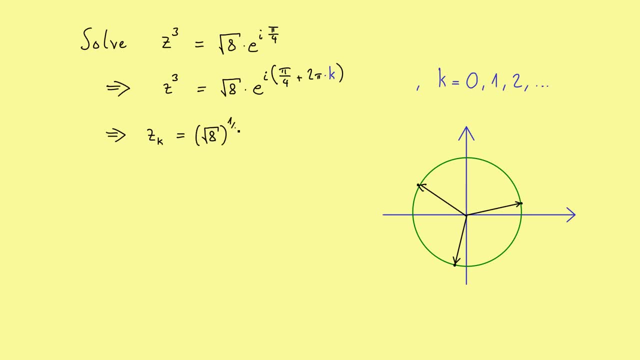 First we have the square root of 8 to the power 1 over 3.. And then the exponential function to the power 1 over 3.. However, this simply means that we multiply this exponent with 1 over 3.. Okay, so let's rephrase that a little bit even more. 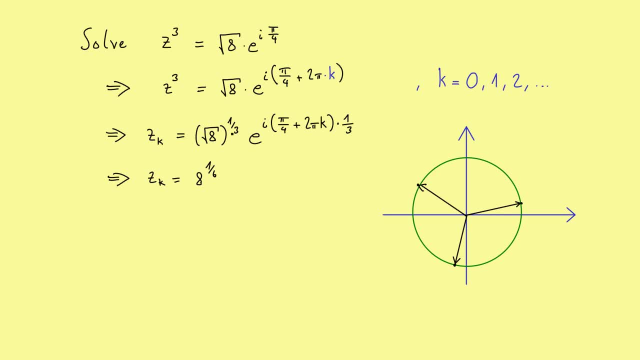 So we can write the 8 to the power 1 over 6. So combine the square root with the 1 over 3. And the same way here we do the multiplication. So we have pi over 12 plus, and there we have 2 over. 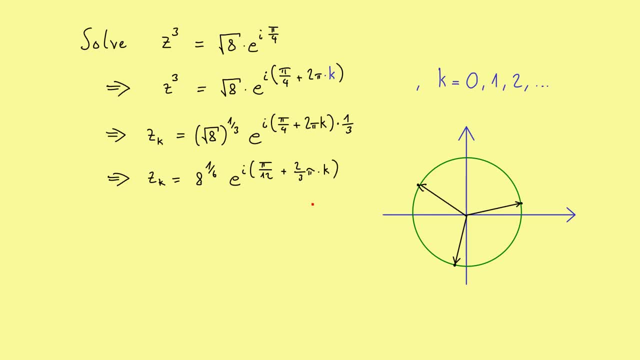 3 pi times k. Well, and here you should immediately recognize Our 2 over 3 pi is exactly our 120 degree. We saw earlier in our circle here And maybe you also recognize our first solution here. This is pi over 12. So 15 degree. 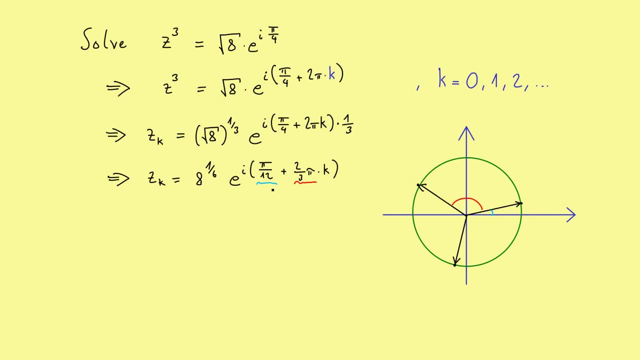 This is the angle here And this makes totally sense, Because now, if you go to the power 3. You have to add up the angle three times. So three times this angle You end up with, And up by 45 degree, Which is our original angle from the number at the beginning. 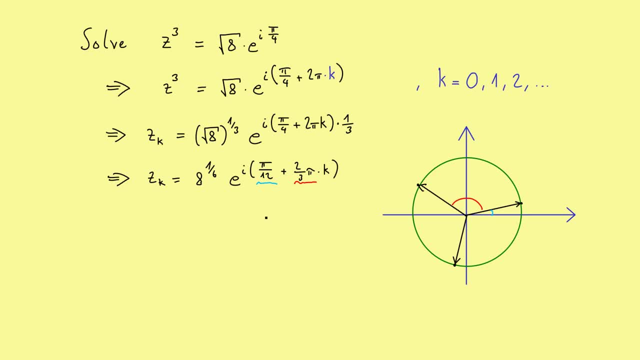 So this is indeed our first solution, And we find it if we put k equal to 0.. Then we find the second solution: if we add 120 degree, So this would be k equal to 1. And if we put k equal to 2. We find the third solution. We could go further, but then you see. 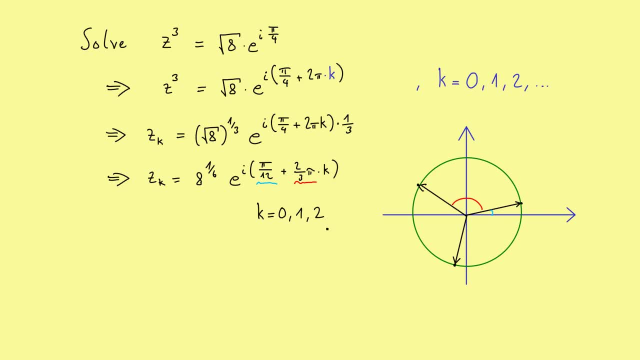 We don't find any new numbers. Therefore we can stop here with k equals to 2.. Okay, so all this we should put in a tidy solution in the end. So the first solution: z 0 is 8 to the power 1 over 6. Which is just the square root of 2.. 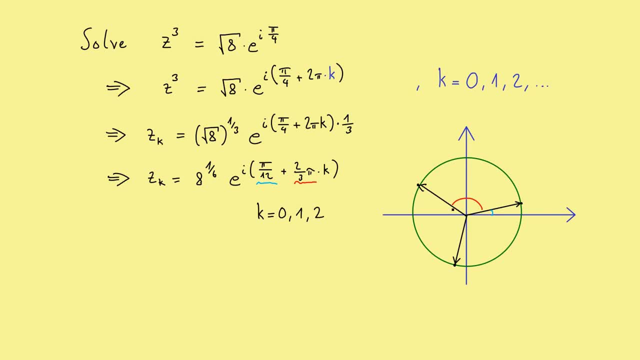 And if we put k equal to 2, we find the third solution. We could go further, but then, you see, we don't find any new numbers. Therefore, we can stop here with k equals to 2.. Okay, so all this we should put in a tidy solution in the end. 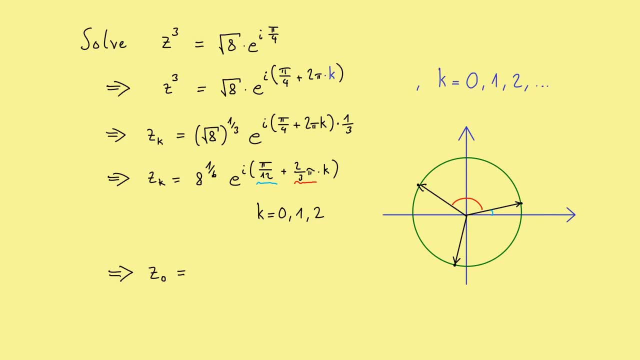 So the first solution- z0, is 8 to the power, 1 over 6, which is just the square root of 2.. That is what you can calculate, But remember this is just the radius of the whole circle here. 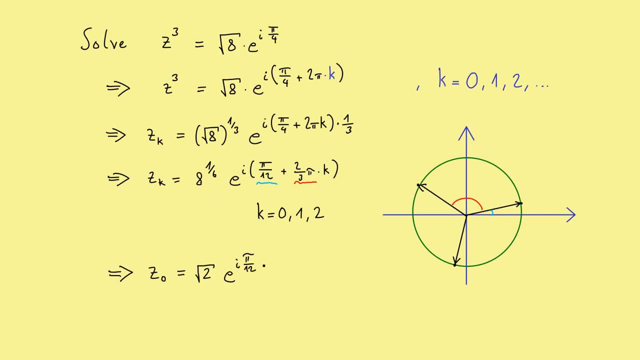 And as the first solution we have the angle Pi over 12 plus 0.. For the second solution, z1,, we have still the same absolute value, but then e to the power i, and now pi over 12 plus 2 over 3 pi. 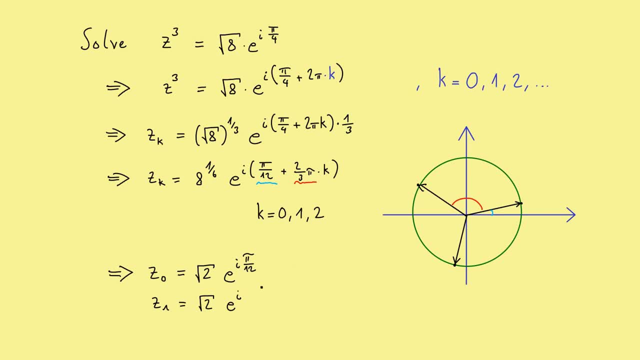 But this one is just 8 over 12 pi. so in sum we have 9 over 12 pi. Then the same holds for the third solution: still the same absolute value, but now we have 9 over 12 pi. So we have again to add 8 over 12 pi, which means we have 17 over 12.. 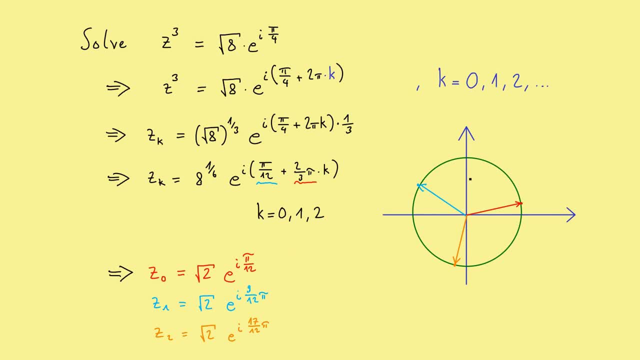 Now using some colors. you now see the solutions in the complex plane, And first solution with the small angle. then we add up the 120 degree, find the second solution and the same way the third solution. I strongly advise you to do that after your calculation. 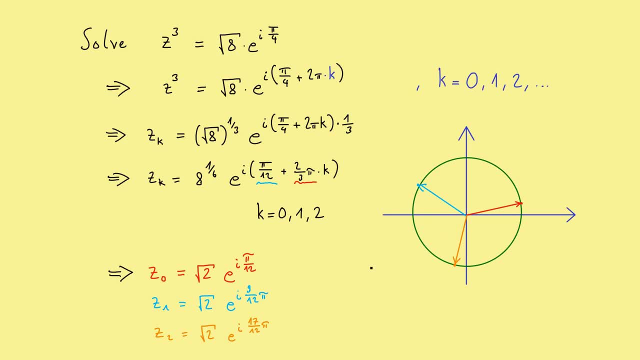 So draw a short scale So that you can sketch with your solutions to see if the solutions divide the circle indeed into equal parts. Okay, and the same way. the same thing works for higher powers, For example. now you should know how to solve z to the power of 4 equals to a complex number on the right. 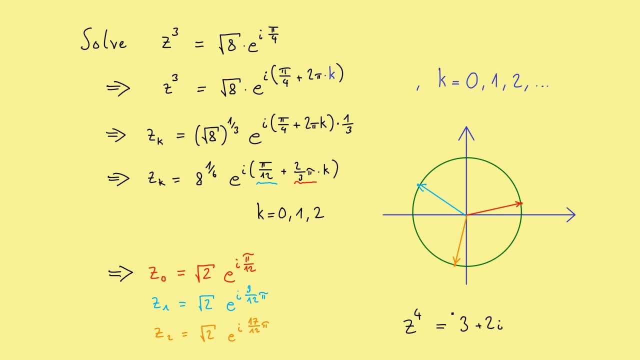 So, for example, 3 plus 2i, First we write this number in the exponential form and then do this scheme here, And then you find the radius and the first angle for the first solution. Now, because you know the power, you already know the angle between two solutions. 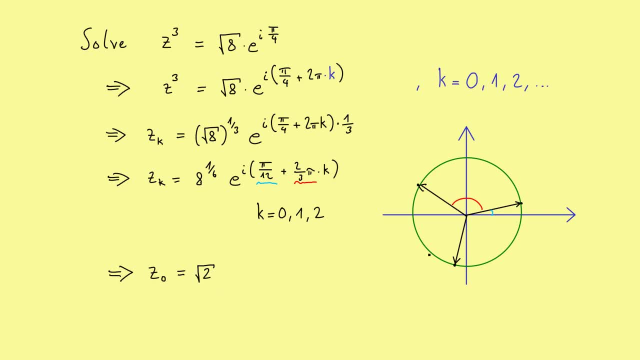 That is what you can calculate. But remember, this is just the radius of the whole circle. here, And as the first solution we have the angle pi over 12. Plus 0.. For the second solution, z 1. We have still the same absolute value. 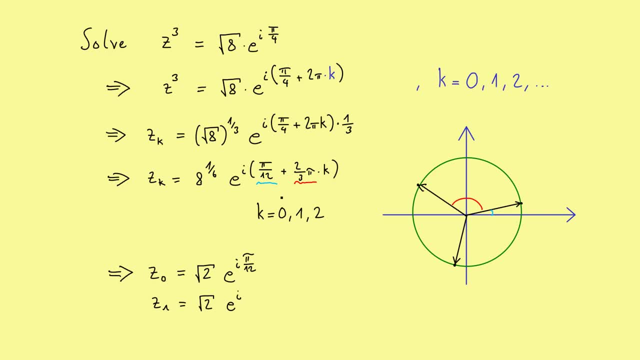 But then e to the power i, And now pi over 12 plus 2 over 3 pi, But this one is just 8 over 12 pi. So in sum we have 9 over 12 pi. Then the same holds for the third solution. 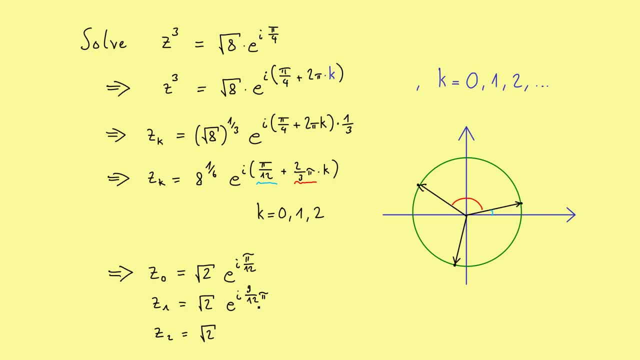 Still the same absolute value, But now we have again Two absolute values. We add 8 over 12 pi, Which means we have 17 over 12.. Now, using some colors, You now see the solutions in the complex plane And first solution with the small angle. 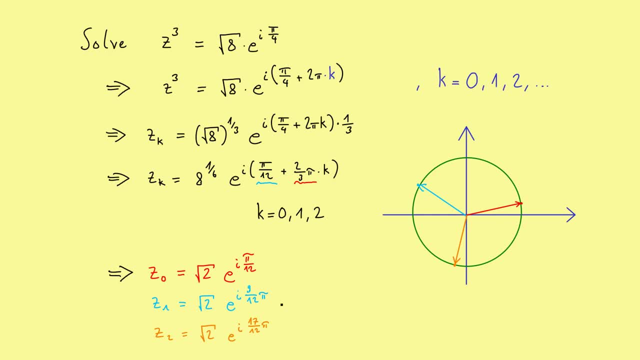 Then we add up the 120 degree, Find the second solution And the same way the third solution. I strongly advise you to do that after your calculation. So draw a short sketch With your solutions To see if the solutions divide the circle indeed into equal parts. 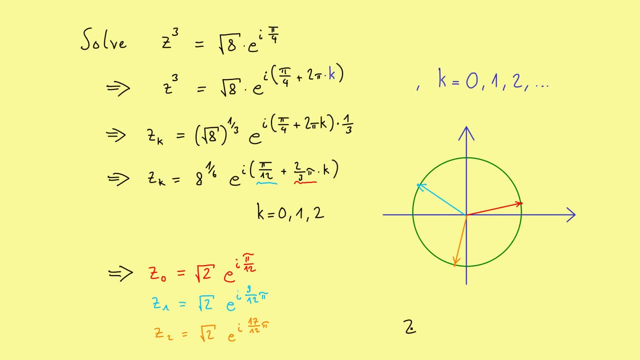 Okay, and the same way. The same thing works for higher powers, For example. Now you should know how to solve Z to the power 4. Equals to a complex number on the right, So for example, 3 plus 2i. 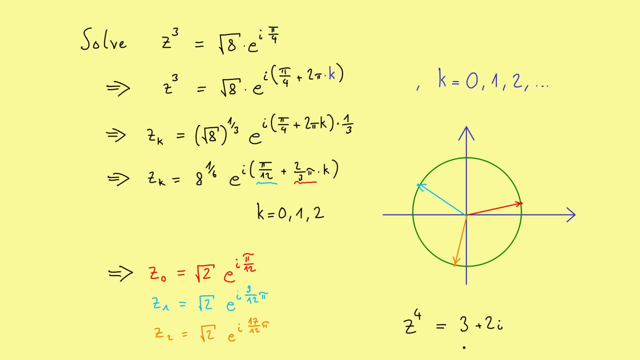 First rewrite this number in the exponential form And then do this scheme here, And then you find the radius And the first angle for the first solution. Now, because you know the power, You already know the angle between two solutions, You know you need four equal parts in the circle. 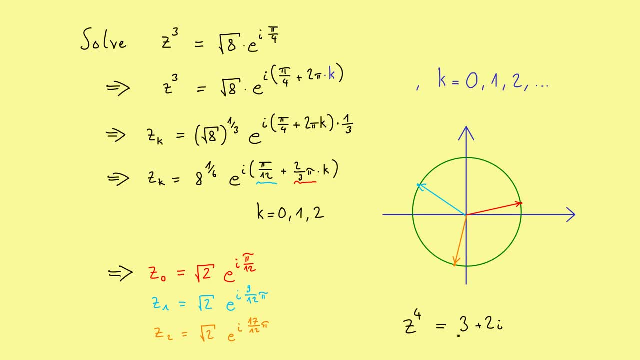 So the angle is 90 degree. This means, with the one exception, That the right hand side is equal to 0.. You always find exactly four solutions For your equation On this circle, Or in other words, If the right hand side is not 0..